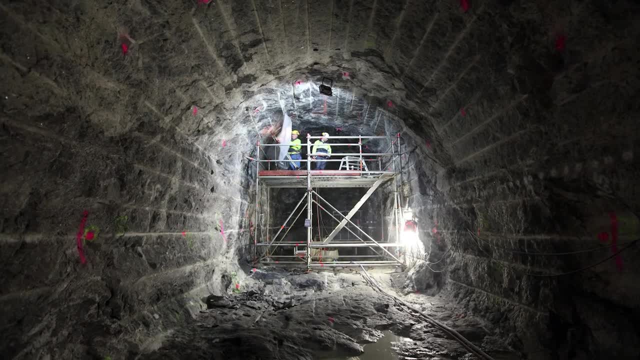 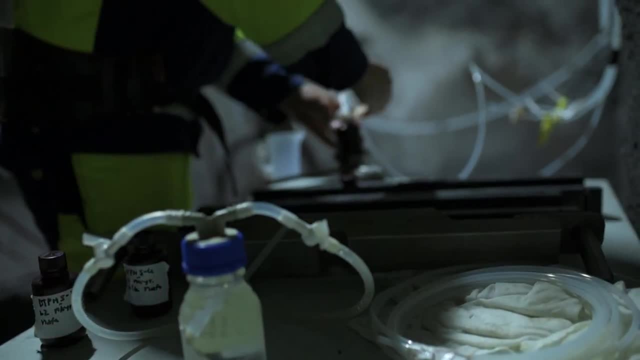 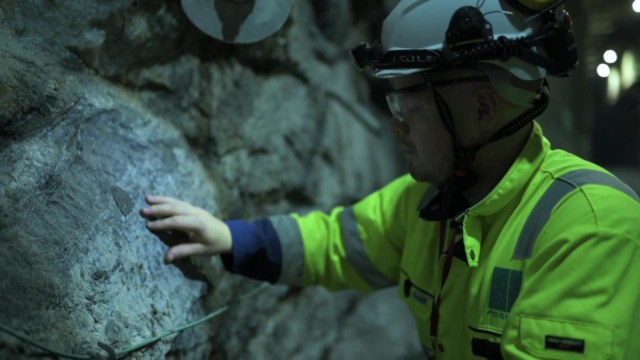 until the radioactive elements inside decay to acceptable levels. It's important to keep water from carrying radionuclides back to the surface, a dangerous scenario for ecosystems and human health. So Ankkolo relies on a series of barriers to keep the copper casks safe. 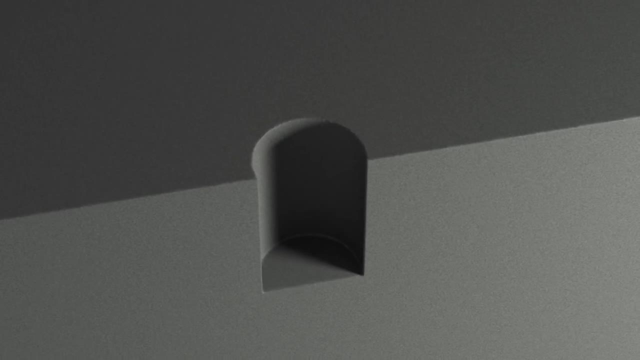 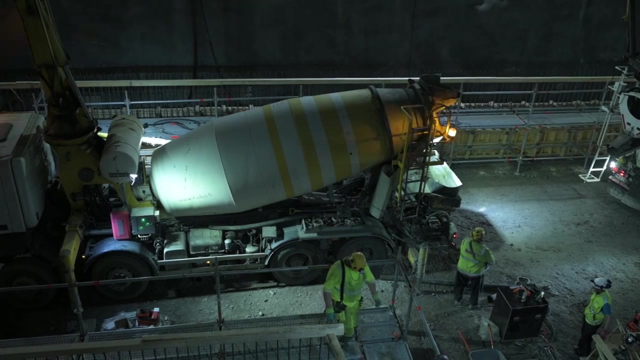 The first barrier is the rock itself: Hard crystalline rocks that have few pore spaces and are nearly impervious to water. Polsiva, the Finnish waste company excavating Ankkolo, mapped the cracks as its workers dug and built the repository. 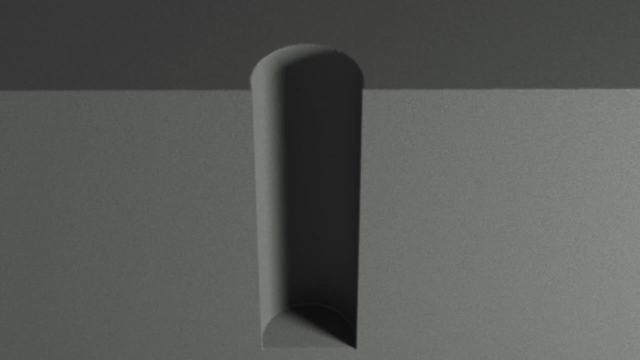 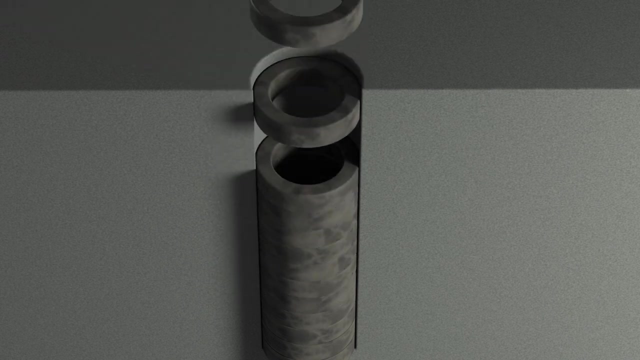 a method to keep them from becoming conduits for water. A second barrier is bentonite, a water-absorbing clay that will surround the casks and plug the burial holes. The bentonite will also block microbes from reaching the casks and speeding up corrosion processes. 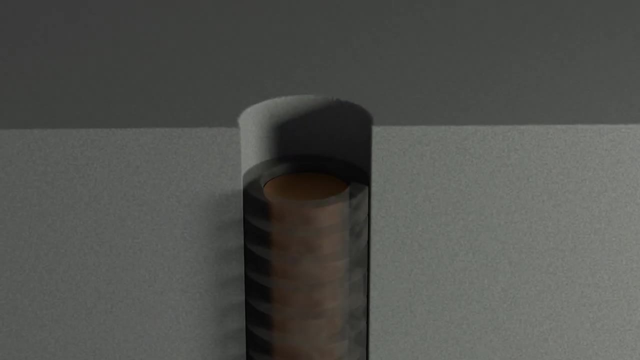 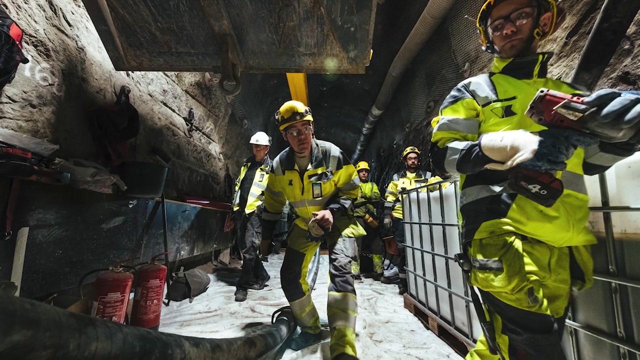 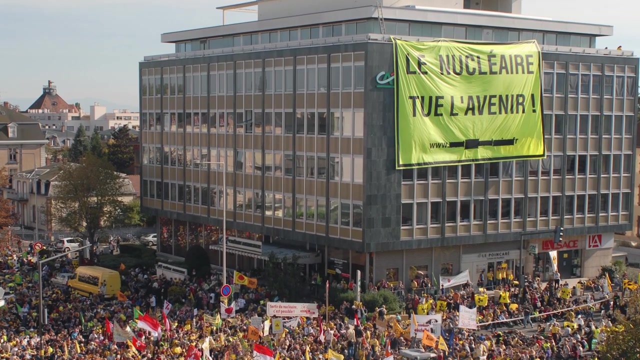 Finally, there's the copper itself. Polsiva says it won't corrode in what little water there might be at such depth, because it's oxygen-free. Ankkolo is not just a technological tour de force. It's a model for navigating controversy In France, the United Kingdom. 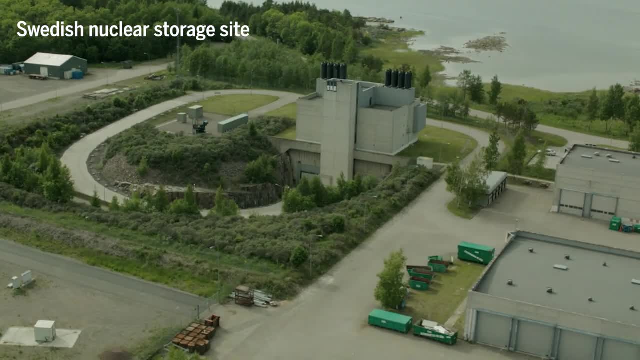 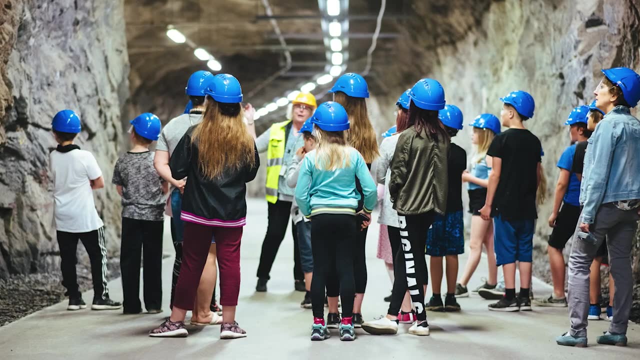 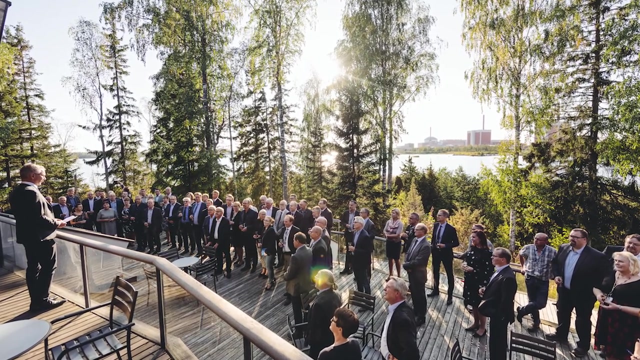 and Sweden. deep nuclear waste repositories have been delayed or thwarted by public opposition. Experts say Polsiva and the Finnish government were better at engaging with residents of Eorajoki, the town closest to Ankkolo. Finnish law gave the municipality a veto in the siting process. 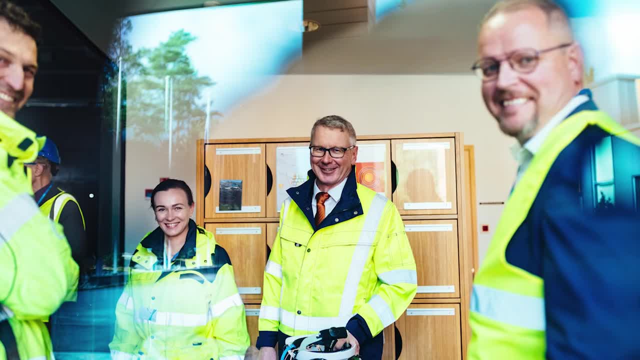 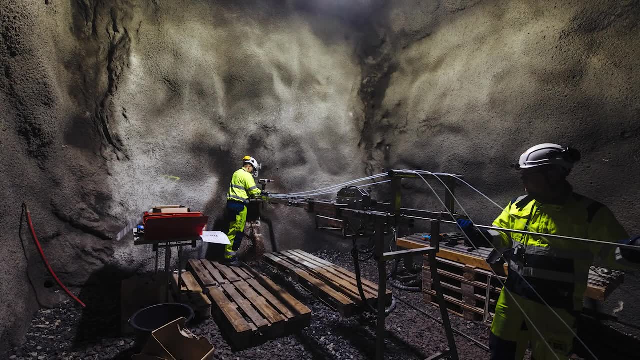 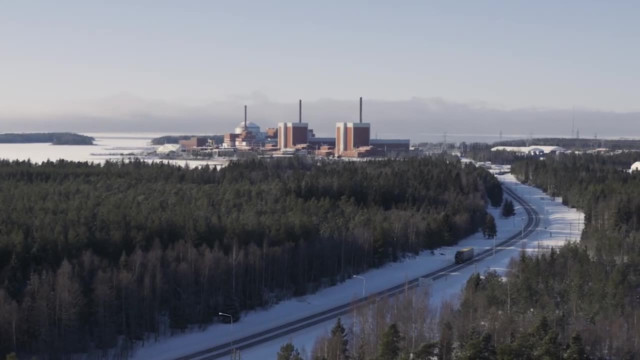 and the company dangled the promise of jobs and tax income, as well as funding a new senior center. Culture could be another reason for Ankkolo's success. Finns trust scientific expertise in state institutions like the nation's nuclear regulator. The lack of state-level politics in 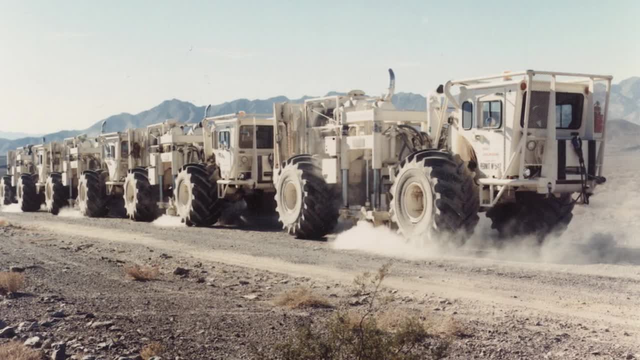 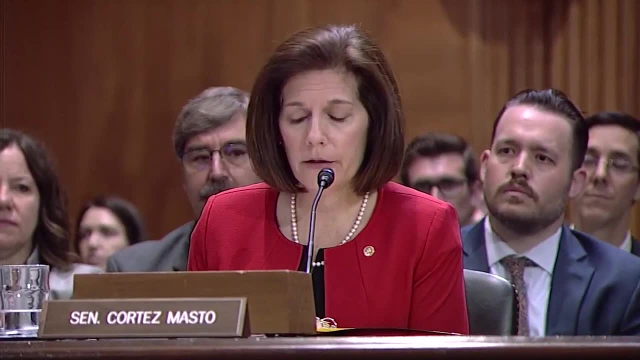 Finland presents another advantage. In the United States, the Department of Energy's long-standing desire to build a repository at Yucca Mountain was thwarted because of antagonism from Nevada politicians To discuss the legislative draft before you and our opposition to Yucca Mountain. 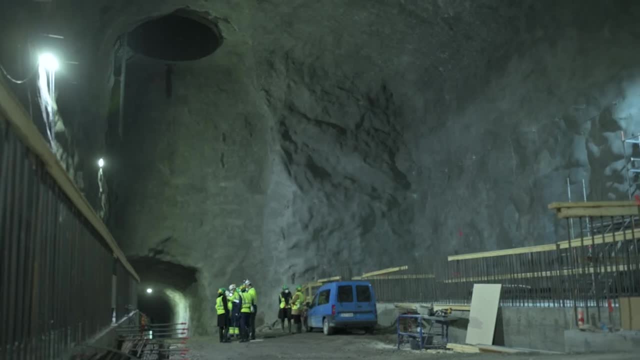 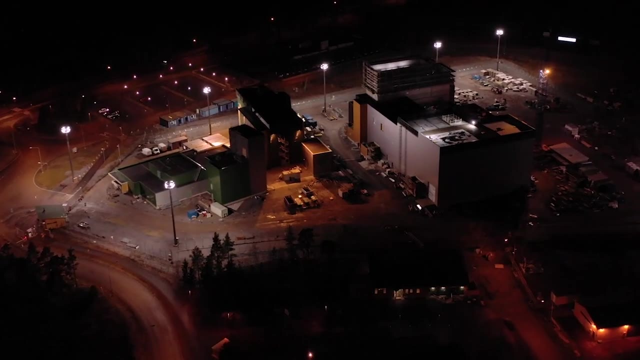 Sometime around the year 2120, after Ankkolo entombed 6,500 tons of waste, all of the access tunnels will be backfilled and sealed up. Surface structures will be dismantled. no sign of the repository will remain But deep underground.